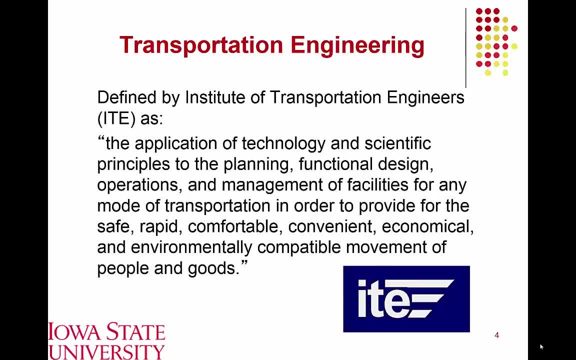 as quickly as possible. The secondary concern there is safety, So we're trying to minimize the likelihood of crashes occurring, And if a crash does occur, we'd like to mitigate its severity. And then we have a variety of complementary concerns as well, which could include comfort. 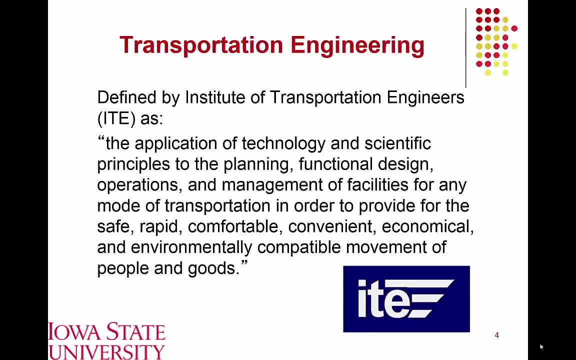 from a road user standpoint, convenience access to transportation systems, how economical these are from the road user standpoint, and then also looking at any potential adverse environmental impacts and trying to mitigate their consequences as well. So as transportation engineers, we are generally trying to. 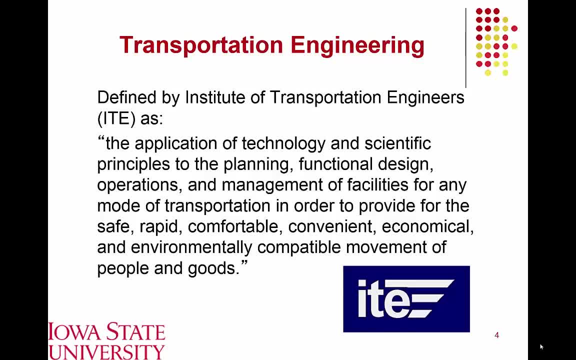 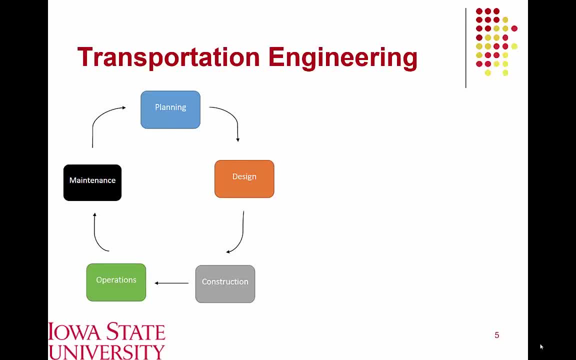 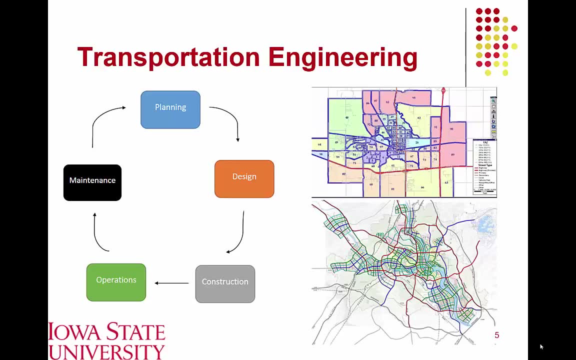 simultaneously accomplish this wide range of goals, and that's what we'll be covering as a part of this course. And so, when we talk about transportation engineering, there are essentially five general phases or activities involved with transportation engineering. The first one is the transportation engineering, And so those would include, at the highest level, planning activities. 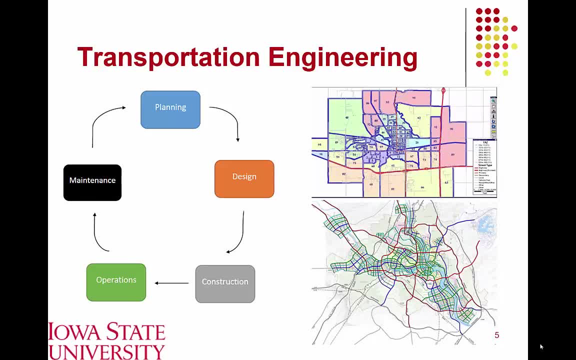 So, from a road agency standpoint, we'd like to be able to put together an inventory of our road network, what facilities we have available to us and what's included in those facilities, as well as what their condition is. So the quality of the pavement on a roadway, how well a roadway. 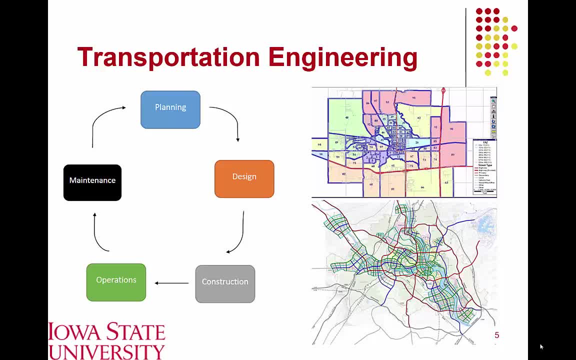 link is performing from an operational standpoint, how many crashes occur on that segment and what are the status of the various features associated with that roadway network. And if we have a good idea of what our system looks like currently and what it's projected to look like moving forward, we can then use 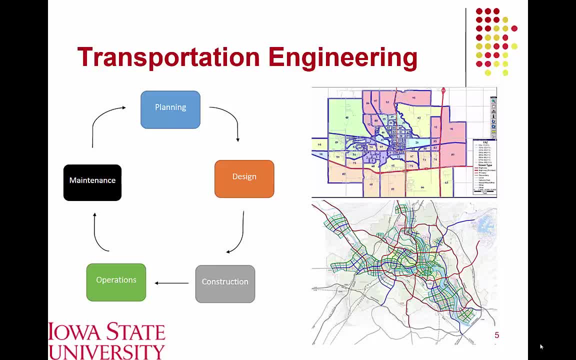 a series of analytical models to try to project how system performance will vary over time, And from that we can determine where there are weaknesses or areas for improvement in our system and then we can plan projects and programs accordingly. So once we've determined that, 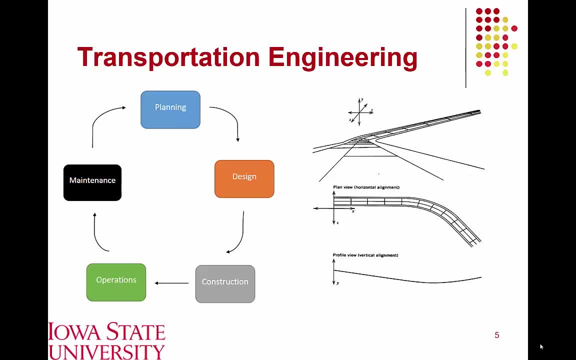 a project is necessary. we would then go through some sort of design process, and the most general example is horizontal and vertical alignment. So designing how the curves align on a roadway would be one example of design. And once that design has been completed, 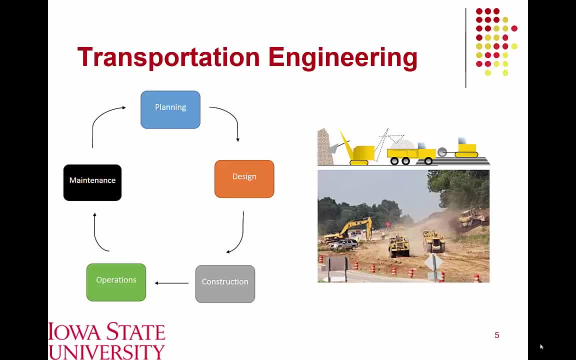 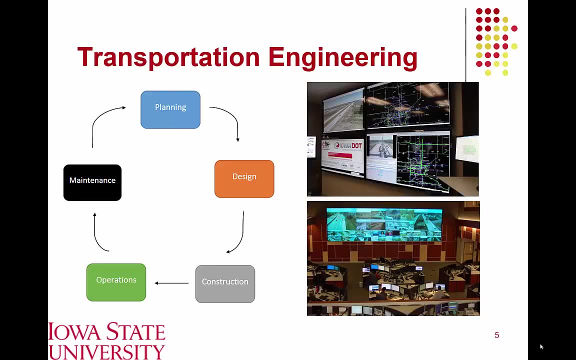 going out and then actually constructing that facility, And so a lot of this would be covered in complementary classes in the construction engineering area, but we'll at least talk in generalities about how construction fits into the bigger picture. And then, once that road is actually put into operation, transportation agencies are. 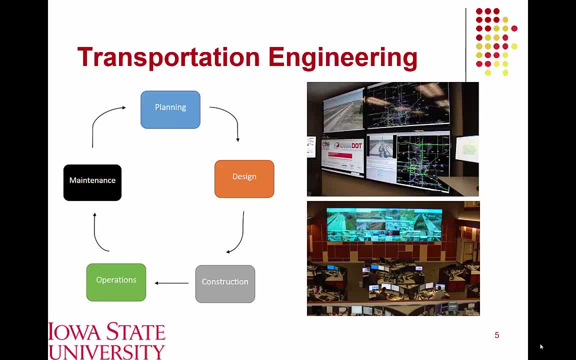 as I mentioned, currently investing extensive efforts to provide essentially real-time monitoring of the performance of the systems or how well it's operating, which is where the term operations comes from. So what we see right here in this diagram, these are just snapshots from a 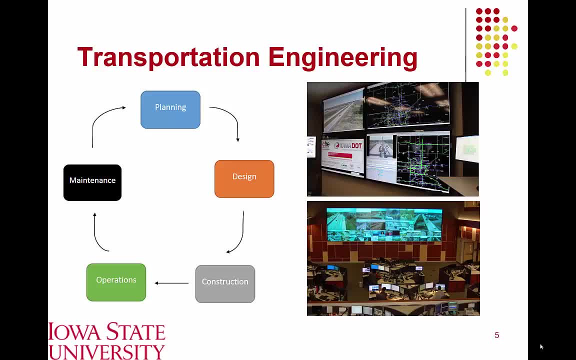 few what we refer to as traffic operation centers, Generally DOTs, just like the Iowa DOT here in the state, are providing real-time monitoring of the freeway network and many of the other major arterials that are under the control of those municipalities, and so we're able to collect real-time data on traffic speeds, traffic volumes. 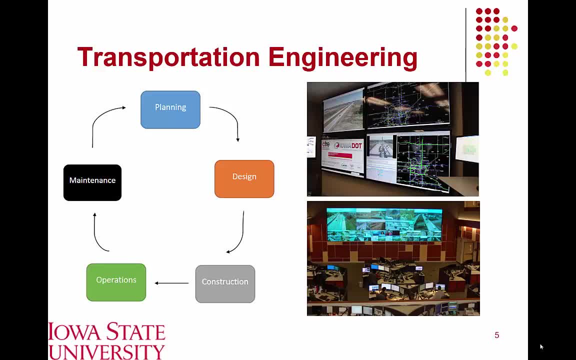 assess whether there are traffic crashes or other incidents that are affecting performance of road facilities, and then we can create proactive response in the event of some sort of issues with the road network, whether that relates to a work zone, for example, or a vehicle breaking down on the side of the road And then going beyond operations. 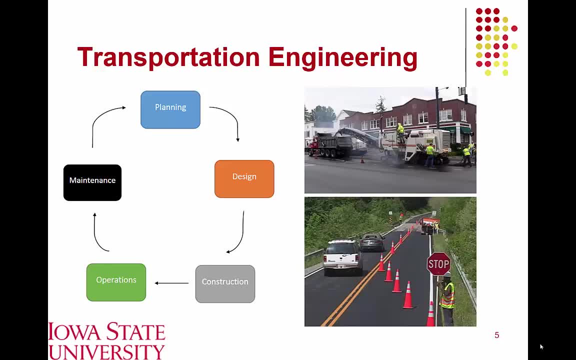 we're also concerned with maintenance, both short-term and long-term, and we're also concerned with the use of the road network, So we're able to collect real-time data on traffic speeds. so, long-term, we're talking largely about construction projects similar to what we had. 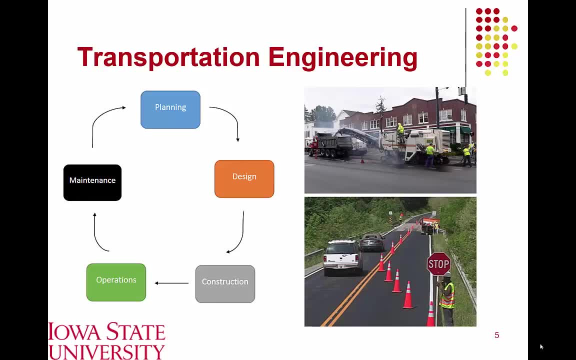 discussed previously, how frequently roads need to be maintained, what exactly is involved in those maintenance activities, and then also shorter duration maintenance, if we need to go out and do some quick fixes, pothole repairs, things of that nature- And so there's a wide range of 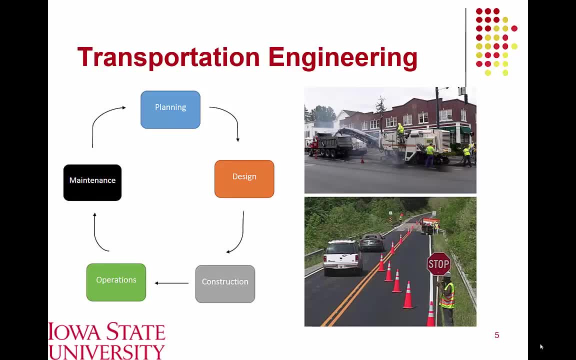 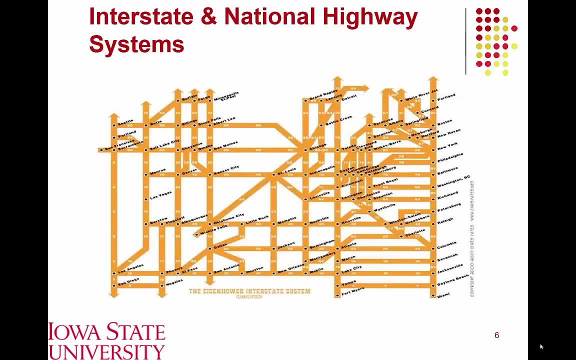 different activities that are involved in transportation engineering and, as a part of this course, we'll provide some level of coverage of various phases of these activities. And one question that arises often is what is the role of the road network and what are some of the? 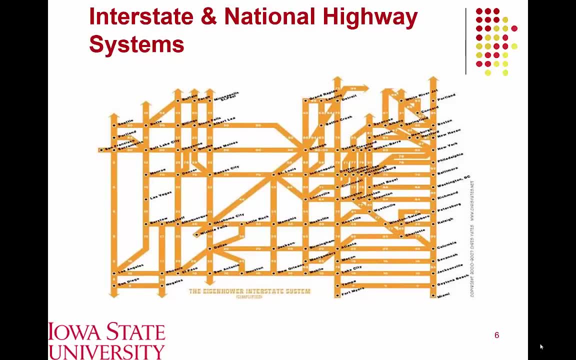 things that we can do to make sure that the road network is a good place to be, And so what we see right here, this is just a schematic map that outlines the interstate highway system, And so what you see here: we've got a series of high-speed roadways, or the interstates which 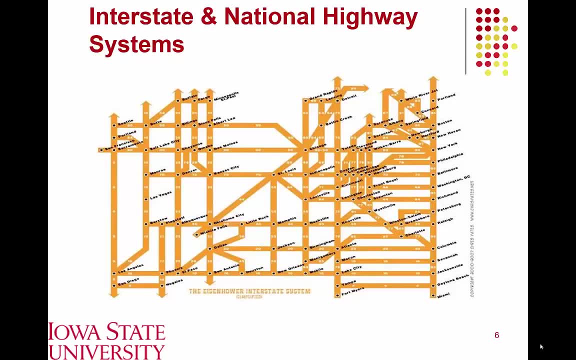 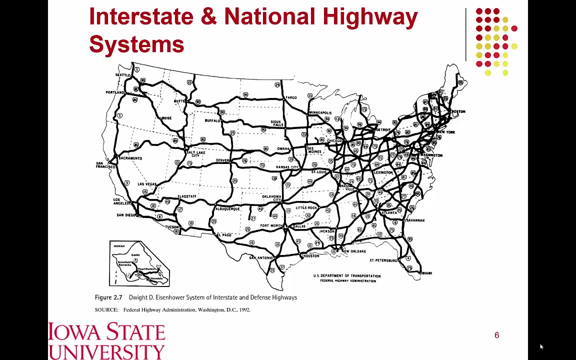 connect large cities across the country basically. So this isn't to scale here, but this is providing us a nice simplistic version of each of these various interstates and where they run to and from, And so the Eisenhower Interstate System was actually the largest public works project in the history of. 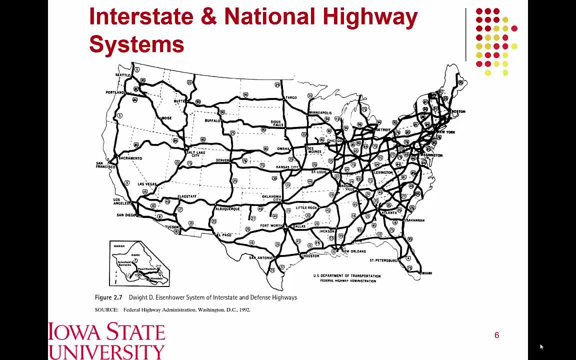 the world, And so this was completed over a series of several decades And, as you can see, it connects. virtually every major city in the United States can be accessed by these interstate facilities, And subsequent to that, we've got a complementary road network as well. 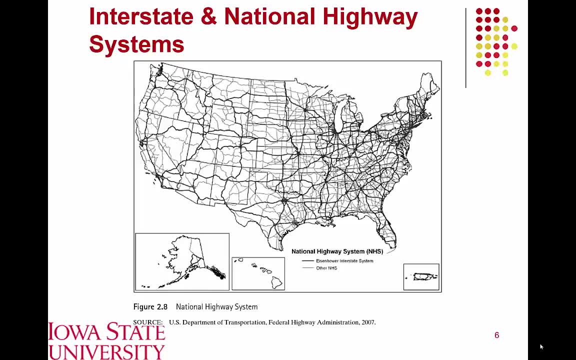 which is referred to as the National Highway System, which includes the Eisenhower Interstate System as well as any other highways of national significance. So it includes the interstates, it includes any US routes and it also includes a large number of state-maintained highways as well. 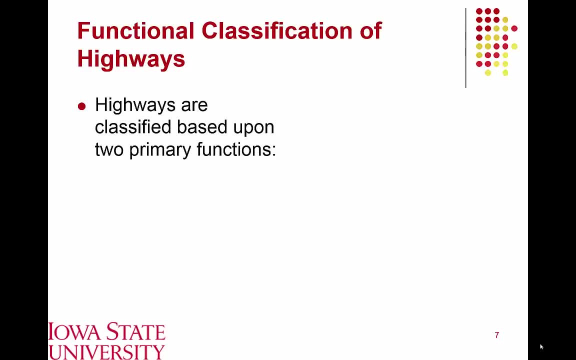 And so, when we look at these roadways, highways are generally designed so that they can accommodate two primary functions, and those functions are mobility and accessibility. So you can look at any type of road and assess its mobility, which is measuring its ability to provide continuous high-speed travel. 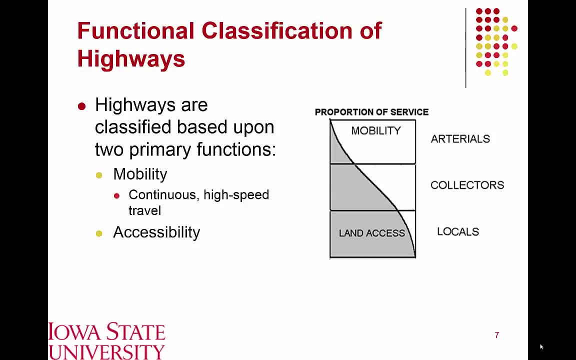 So people would be able to travel on a road that has high mobility, because they can move quickly, with minimum time, from one location to another. But in combination with that, our road system also needs to provide for access. So accessibility refers to the roadways' ability to actually get you to your destination endpoint, for example. 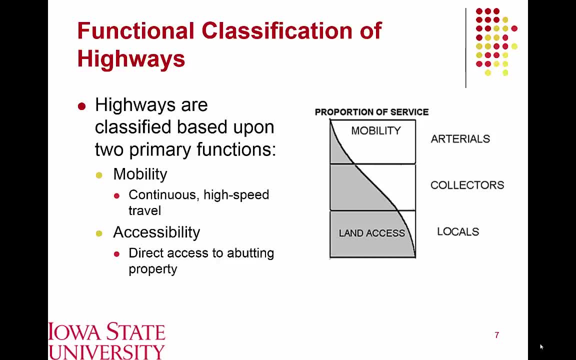 So a parking lot or the driveway to your house. And if we look at different types of road facilities- interstates, for example- would provide very high levels of mobility. You can travel as fast as you would like up to a practical upper limit, but very low access. 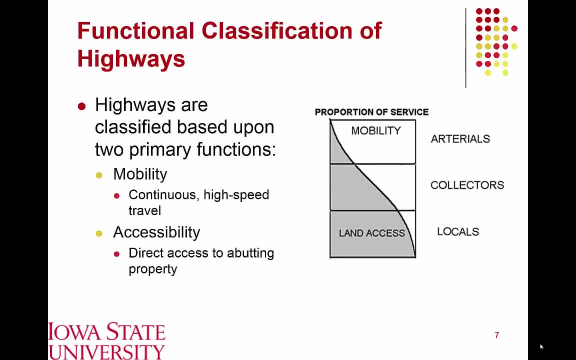 You can't get into your driveway directly from an interstate, for example, Whereas lower class facilities like your local street network will have very good access. you can get door-to-door, but speeds and mobility as a function of that are much, much lower. 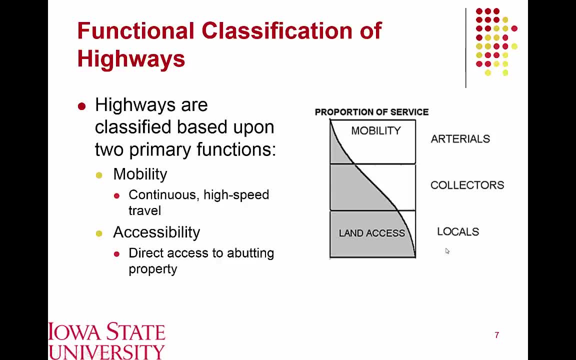 And so, as you see in the diagram right here, there's a clear tradeoff between mobility and access, and we'll operate different types of facilities so that they're either primarily satisfying mobility versus accessibility, versus a combination of the two, as we'll cover in a few of our subsequent lectures. 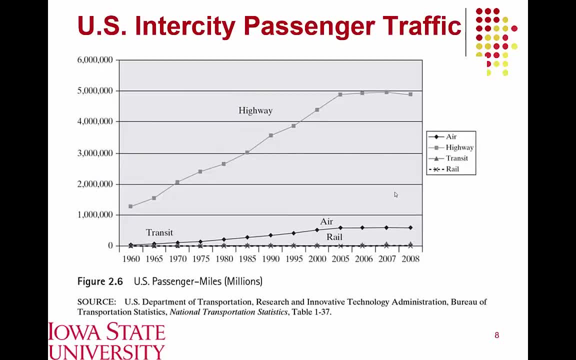 This slide demonstrates recent trends in passenger vehicle traffic. So what we see here, this is intercity passenger traffic. So going from one to the other. So this slide demonstrates recent trends in passenger vehicle traffic. So what we see here, this is intercity passenger traffic. 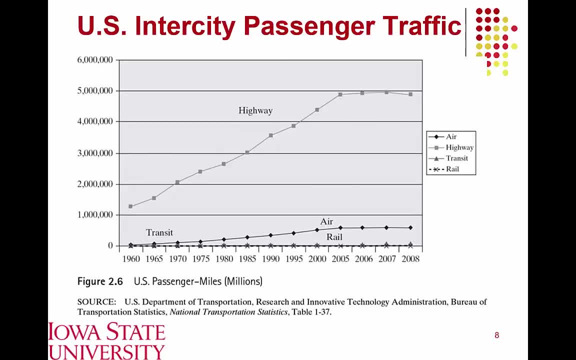 So going from one city to another, long-distance travel essentially, And what we see on the y-axis here is the number of passenger miles traveled in millions across the United States going back to the 1960s, And we see how that mode share has changed with respect to highway versus air versus rail versus transit. 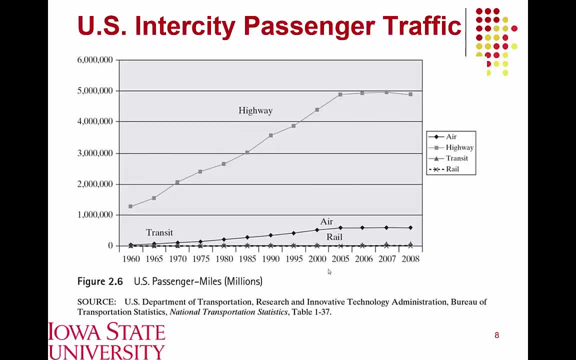 And, unsurprisingly, we've seen relatively stable and low levels of utilization of transit in the rail system. We've seen significant increases in air traffic over the past 40 to 50 years, but they haven't been nearly that of what we've seen in the highway network. 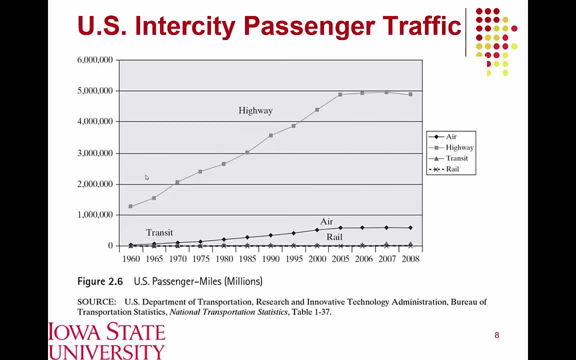 So now we see virtually every household in America has an automobile and we had seen a period of nearly consistent linear growth from the 60s up through roughly 2000.. Now subsequently, over the last 10 years, that traffic has leveled off, as you can see right here. 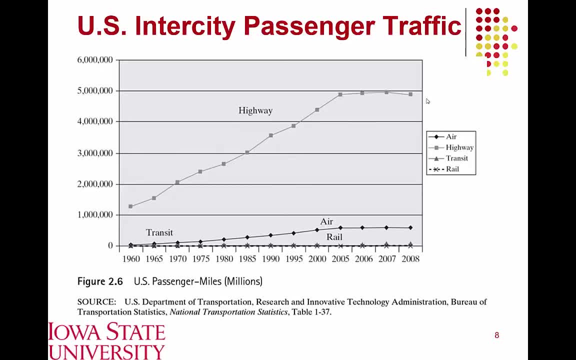 But this drastic growth that we've experienced over time has had a number of repercussions that we're feeling with respect to operation of this transportation system. But this drastic growth that we've experienced over time has had a number of repercussions that we're feeling with respect to operation of this transportation system. 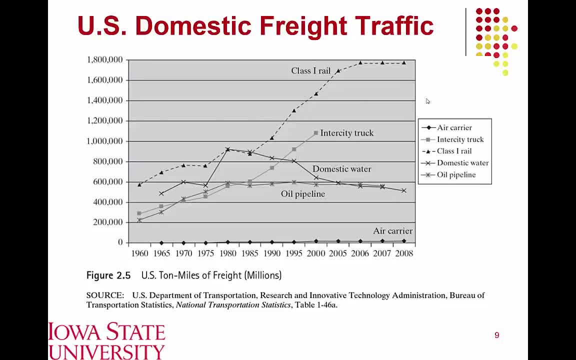 But this drastic growth that we've seen over time has had a number of repercussions that we're feeling with respect to operation of this transportation system, If we look at the freight side of things. so the prior slide demonstrated the movement of persons over long distance. 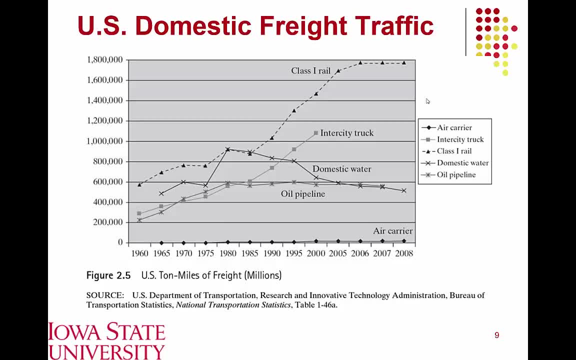 This is demonstrating freight movement And somewhat surprisingly perhaps you'll notice here that the largest share of freight traffic is actually using our rail system, And the primary reason for that is that the rail system is relatively low cost to operate and ship, particularly for very large pieces of cargo. 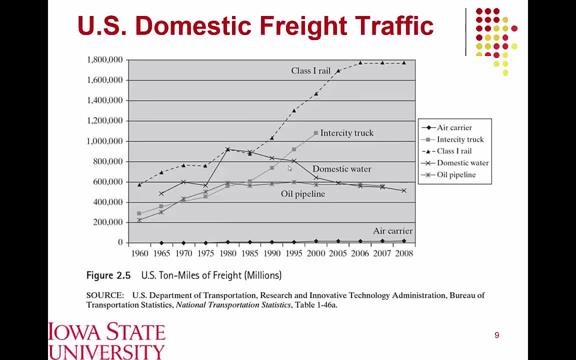 We've seen significant increases in the share of truck traffic, So this would be large commercial vehicles or semi-trucks you would see on the interstate system, for example, And we've seen drops in transport by water and less transport by air as well. 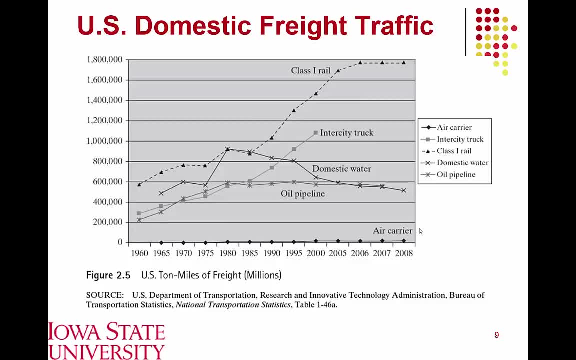 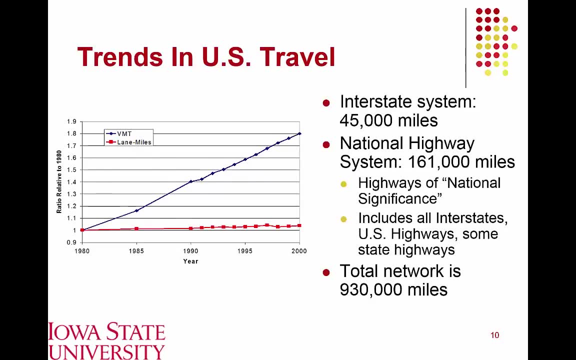 And a lot of that relates to cost and accessibility issues for those respective types of facilities. So, looking at large-scale trends in travel, what we see right here this is just showing us the relative ratio if we compare at five-year increments back to a baseline of 1980.. So looking at large-scale trends in travel, what we see right here, this is just showing us the relative ratio if we compare at five-year increments back to a baseline of 1980.. So looking at large-scale trends in travel, what we see right here, this is just showing us the relative ratio if we compare at five-year increments back to a baseline of 1980..